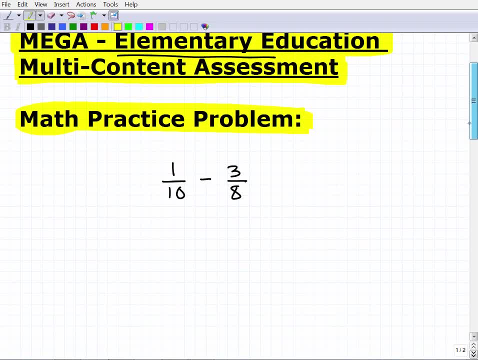 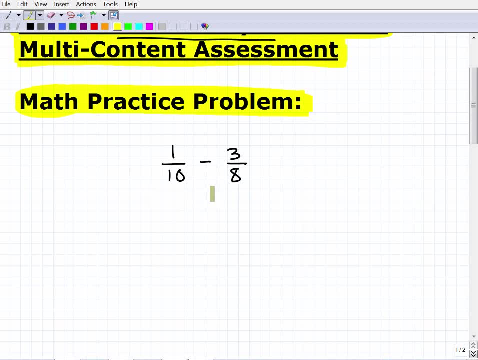 But what I have here for you is kind of a little bit of a pop quiz. So of course you know, at first glance this might seem pretty easy, So that's good. So what I'd like you to do, if you kind of want to play along here for a second, is to pause the video and go ahead. 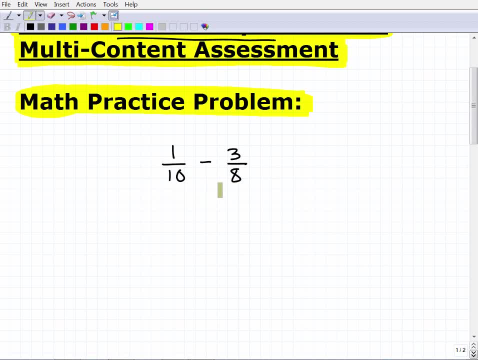 and do this real quick without the course, the aid of a calculator, have your final answer and then I'm going to review it, Then we'll talk about a few other things and we'll kind of go from there. All right, So hopefully you paused the video and 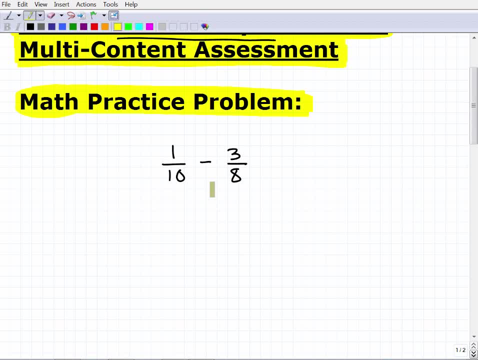 gave this a try, or you just want to continue watching this video. So now, what are we talking about? Well, we're talking about taking this fraction here, Okay, And we have this. Well, we have two fractions. We're going to take the difference, We're going to subtract one fraction. 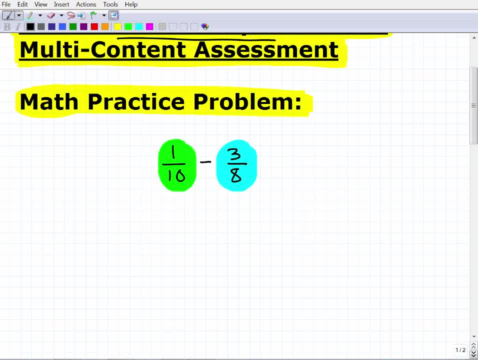 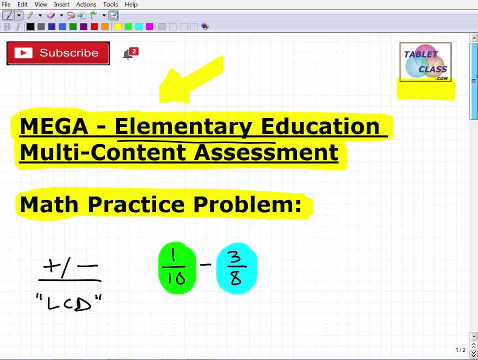 from the other. So just a quick review about fractions here. When we're adding and subtracting fractions, that's when we have to really deal with the LCD. Now one thing before we get going. I made a video some time back on my YouTube channel. I've been on YouTube for 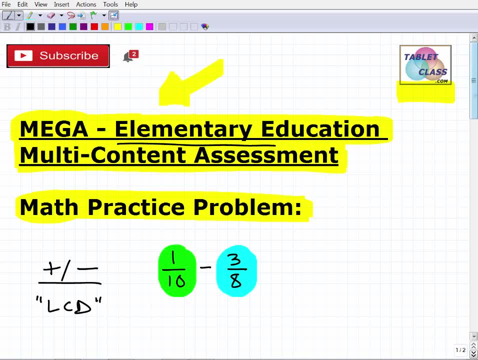 many, many years, And one of the videos that I made was- I can't remember the title exactly, but it had to do with learned fractions. I think it learned fractions in seven minutes And that has hundreds and hundreds of thousands of views. It might be even approaching maybe even you know. 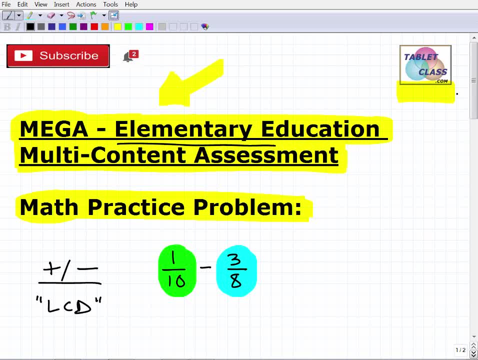 close to a million views, 700,000 views, something like along those lines. So if you're a little bit weak on fractions, you want to check out that particular video. I think that would really help you. It's just a quick crash course on fractions. 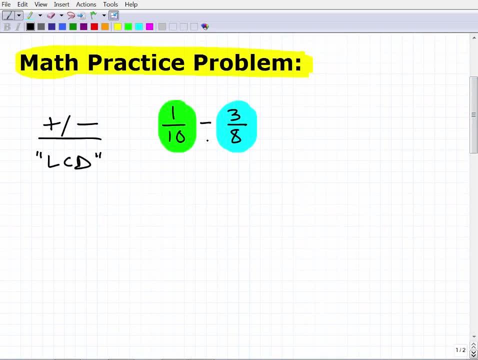 But again, when we're looking at two different fractions, when we're seeing a subtraction or addition operation, that's when we have to think about the LCD. When we're dealing with multiplication and division, this is actually very easy. So just a quick review. 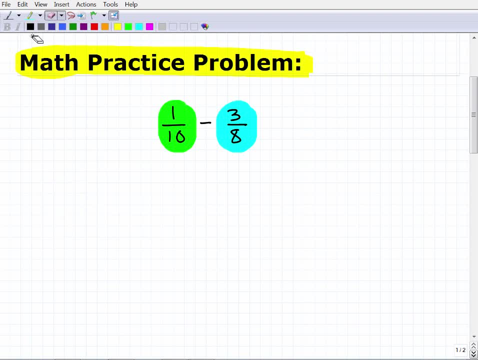 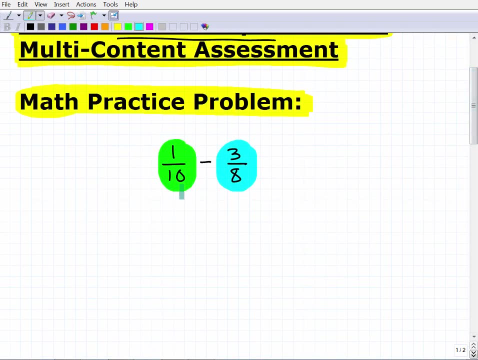 A lot of people see fractions and they'll just automatically start thinking, oh, I've got to deal with the LCD, et cetera, et cetera. Yes, of course you do in subtraction and addition scenarios. Now I'm not going to go through the typical way that you may approach. 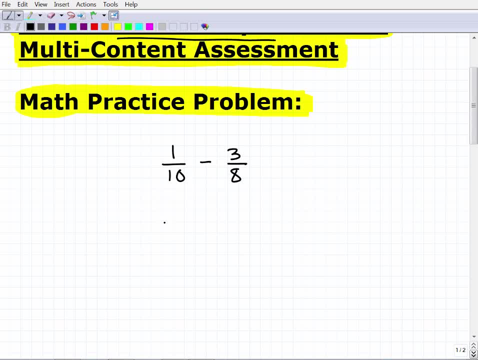 Most people probably would have approached this problem, And that is okay. they're looking for the lowest common denominator. And let's see here: 8 times 5 is 40. So 40, right, would be the lowest common denominator. 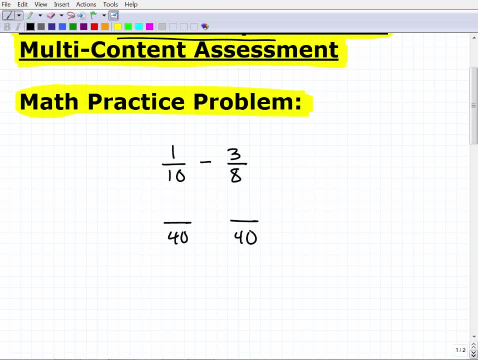 And then we'd go from there. Now, if you did it that way, that's excellent And that's a good way to approach it. What I want to do is teach you a quick method: how to add and subtract fractions. I call this the bow tie method. kind of like a bow tie like this, like someone would wear. 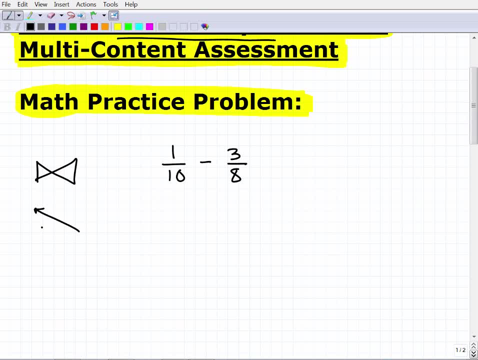 And the reason why I call it the bow tie method is we're going to kind of think of this pattern like this. You kind of see that looks like a bow tie, So let me just show you what I mean. So we're going to multiply this way. 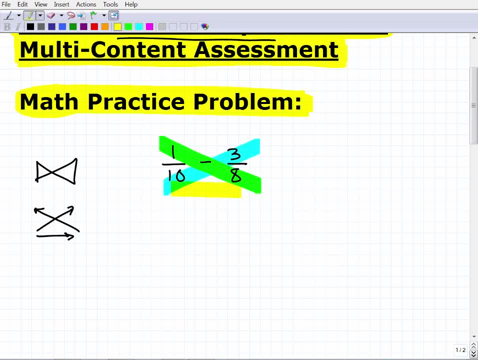 We're going to multiply this way, And then we're going to multiply this way. So let's see how this works, And this is a real handy method of adding and subtracting fractions, especially when we're dealing with algebraic situations. So here is step one. 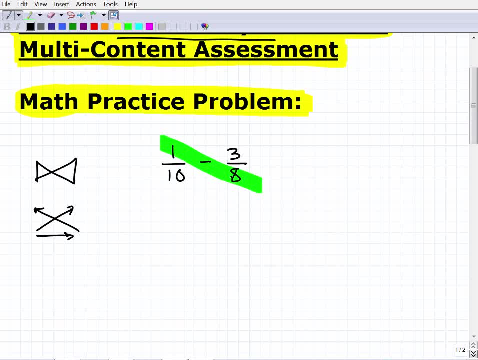 So the first step: we're going to multiply this way, So 1 times 8, we're going to multiply the numbers in this diagonal here, So 1 times 8 is 8.. Now We see that we're dealing with the subtraction scenario. 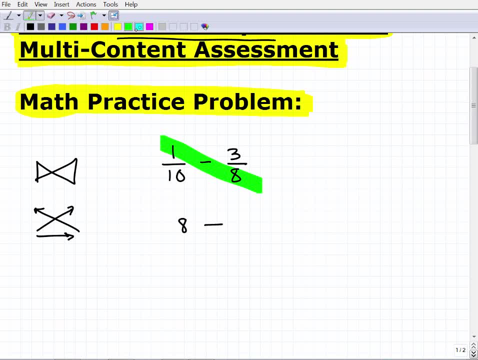 So we're going to put the subtraction operator here Now we're going to multiply this way. OK, so it's always this diagonal, This, this. the steps here are very specific. So the 1 times 8, let me go back here- is going to be the first number. 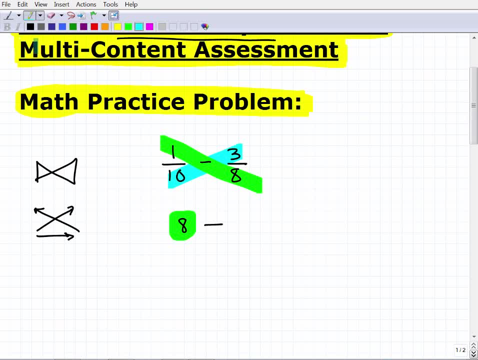 The second number is going to be this diagonal. So 10 times 3 is 30.. OK, so we'll put that here Right. So this direction, this way. here it's going to be the first number. This, the product of these two numbers, is going to be this number. 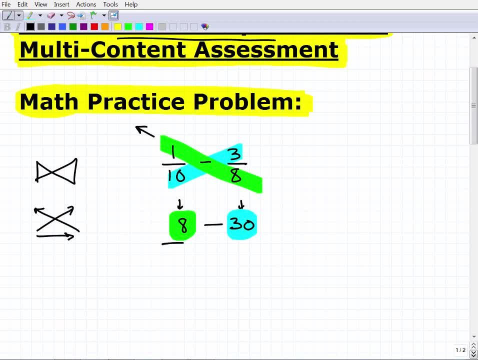 Now this is going to make up our numerator of our answer. Now we're going to put a fraction bar and to get our denominator we're going to go this way. So 10 times 8,, of course, is 80.. 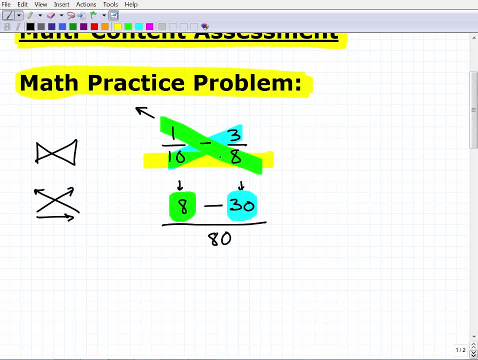 Now we know that the lowest common denominator here It's actually 40.. And here we have a denominator that's 80. Don't worry about that, because we can always reduce this. But this is. I'm going to show you the value of quickly adding or subtracting fractions this way. 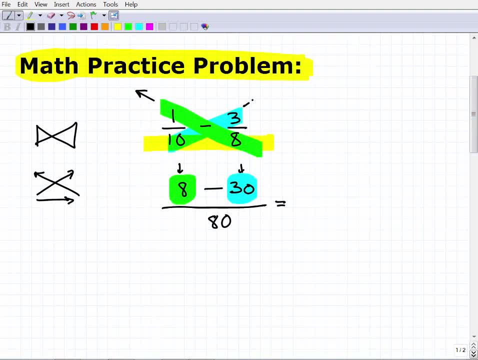 So it's a tool that you definitely want to know. So this is kind of a real bonus. If you didn't know this, I think that you'll walk away with a nice little bonus tool here in a second. So let's go ahead and simplify. 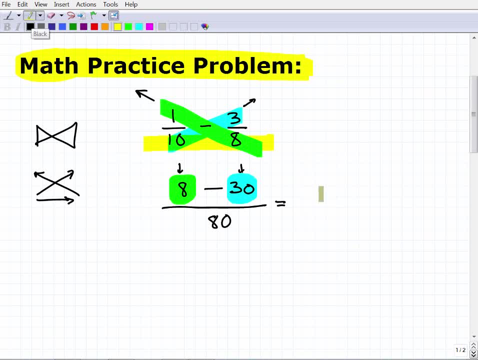 So we have 8 minus 30. So what is that answer? What's 8 minus 30? All right, So hopefully You didn't say 22 and hopefully you said negative 22.. All right, So if you said negative 22,, then that's excellent. 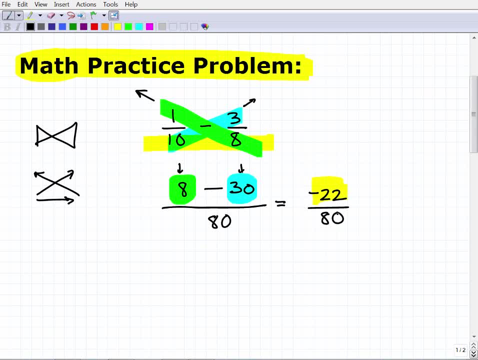 All right, So we have negative 22 over 80. And this is the answer, Okay. However, we want to go ahead and simplify this. So 2 goes into 22,- 11. So this would be a negative 11, and 2 goes into 80,- 40.. 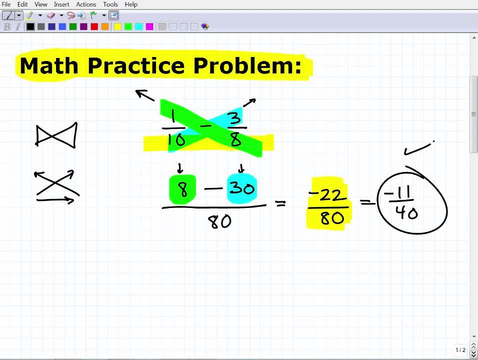 So this would have been our final answer: Negative: 11 over 40.. So if you got that As your answer, but just go ahead and figure out what the lowest common denominator is, Of course that was 40.. What we talked about 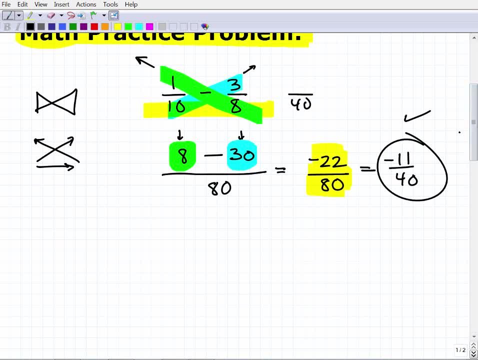 That's excellent, But I wanted to show you this particular method. Now, this is the reason why this method comes in really handy. I'll give you two quick examples. If I said, find find 3 over, let's say, 197 plus 5 over 701.. 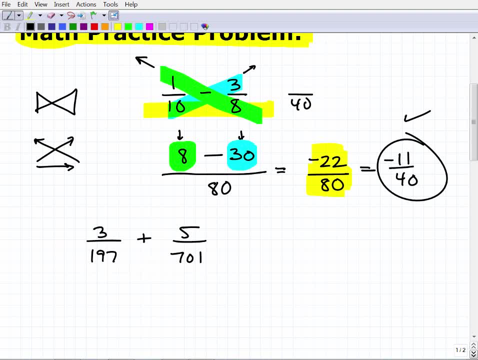 Okay, And you're like: okay, Let me figure this out. Well, you'd first have to try to figure out what is the lowest common denominator. Okay, So what is the LCD? and finding the LCD between these two numbers is pretty easy. 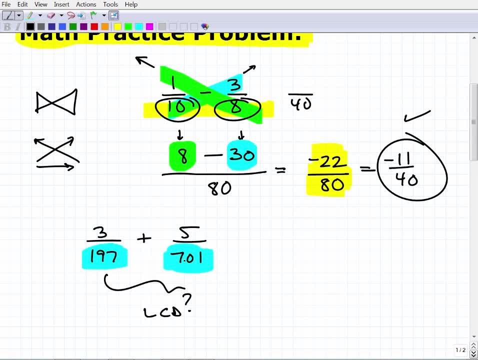 But finding the LCD here? well, that's another separate lesson. So of course I cover all this in my in my full course. But if you didn't want to bother and try to like really go through all the trouble and figure out what is the LCD. 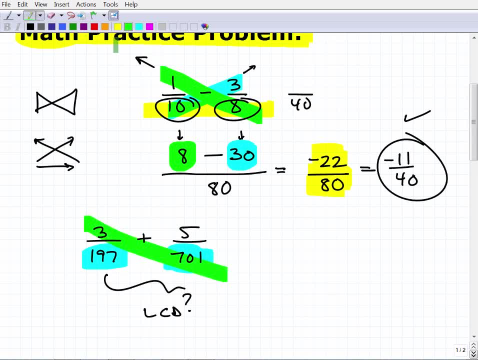 We could simply just Use that bow time method. We can go from: this times these, two times this, this times this, and then we can go- let me use a different color here, This times this. Okay, Just like I did. 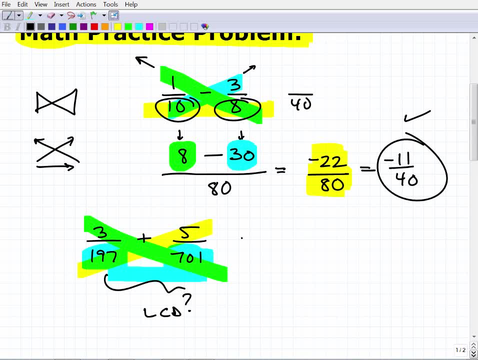 And then you would end up with a big fraction, And then all you'd be left to do is reduce it, And reducing a fraction is much easier than just trying to figure out the LCD. Okay Now, another advantage of knowing this bow time method is, if I gave you this: 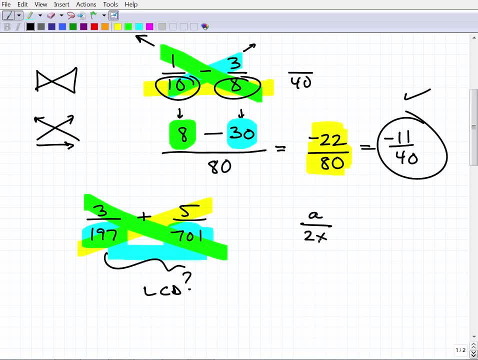 Problem. Let's say I had a over two x plus three over y And I said to simplify that, Well, again, you can use this bow time method. Okay, Let me use these colors. would be this times this, Okay, And then these two products here would make up our numerator and this would be our denominator. 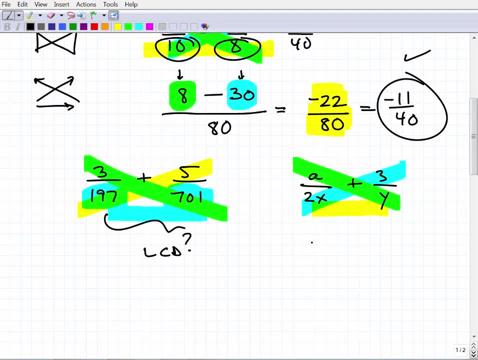 So let me show you how this would work. So a times y is a y plus, right, Because this is a plus problem. Two x times Three would be six x. So this is my numerator and then my denominator would be two x times y or two x y. 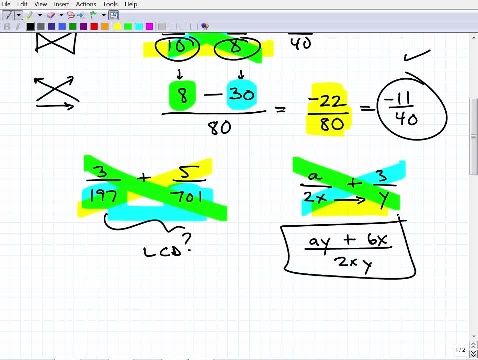 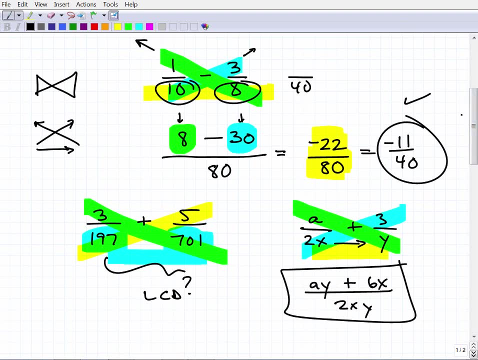 So this particular method of adding or subtracting fractions is really, really powerful. It's definitely something you want to know as a tool when you battle fractions, But anyways, if you got this problem right, particularly the negative part of it, then that's outstanding. 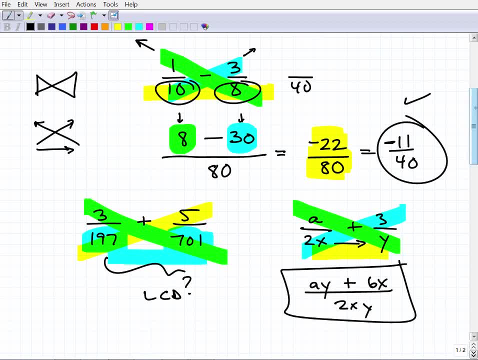 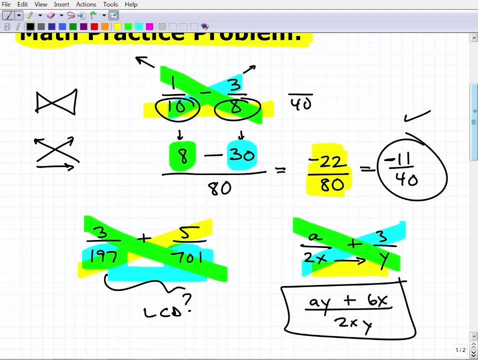 All right, So I don't want to continue on and make this until a full, complete lesson on fractions. Okay, But I did want to at least give you a nice little tip on fractions, if you're still with me to this point of the problem. 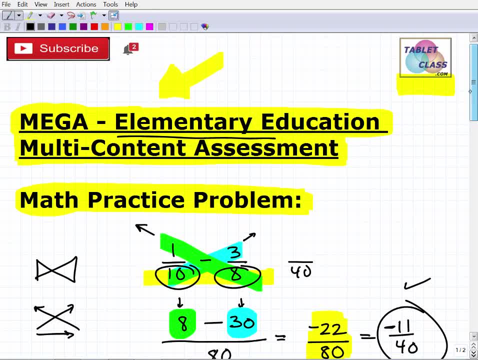 So let's go ahead and wrap it up Again. I'm going to leave the link to my full math prep course for the MEGA Elementary Education Multi-Content Assessment in the description of this video Very comprehensive course. I think you'll like what you'll see there. 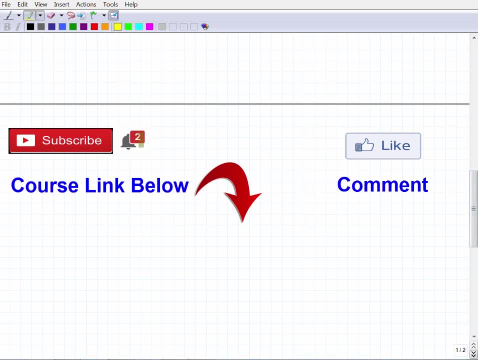 But beyond that, I have been on YouTube at the time of this video for like 12 years. I have hundreds of thousands- actually I think like 13 million- views, well over 100,000, I think 126,000- subscribers at the time of this particular video. 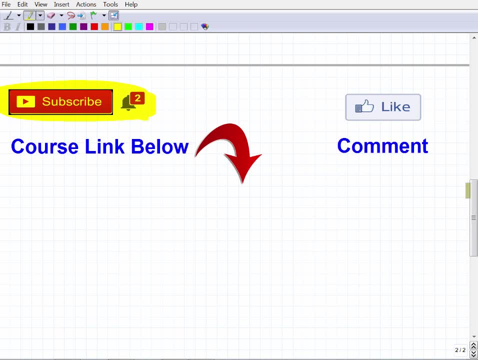 I only say that because to be on this platform for 12 years, you got to be pretty passionate about teaching math and that's what I am right. I'm always posting. I'm always trying to post problems that can, or post little mini lessons. 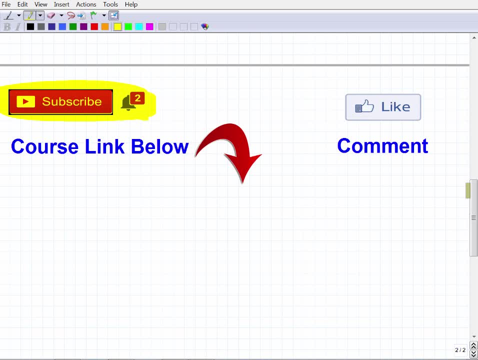 or tutorials or how to solve various different type of problems. So If you like my channel, or even on my channel, there's a lot of video content, if you like my teaching style, that you can use to prepare for this exam. So I encourage you to check that out. 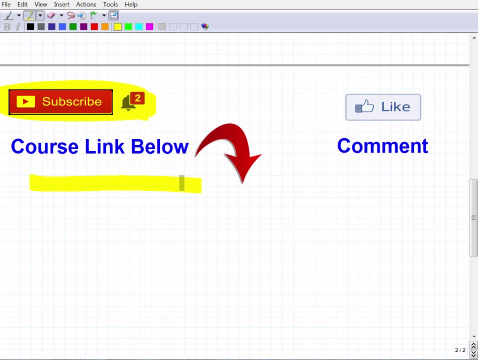 Again, I'm going to leave a link in the description of this video to my full test prep course And if you like this video, definitely appreciate a thumbs up and leave me some feedback. Any feedback is good feedback. I certainly like to hear from fellow teachers. you know, just like you went through that. 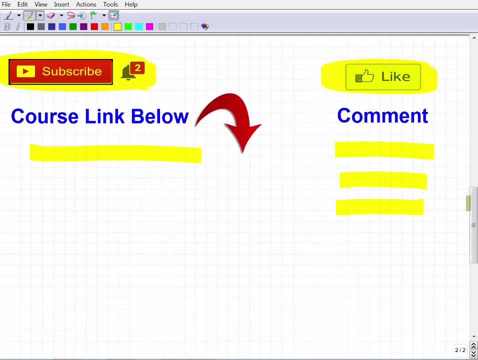 whole process of teaching. If you want to learn more about the process of studying and taking certification exams, I will say this much: When it comes to certification exams or assessments, whatever you want to call it- it doesn't make a difference what state you're in. 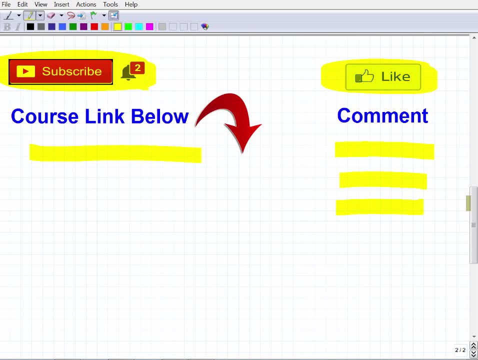 When you're a teacher. the only people really to understand what teachers go through are the teachers themselves. There's a lot of tests, I mean a lot of education you have to have and you have to study really hard for all of these various different certification exams, whether it's elementary school, middle school. 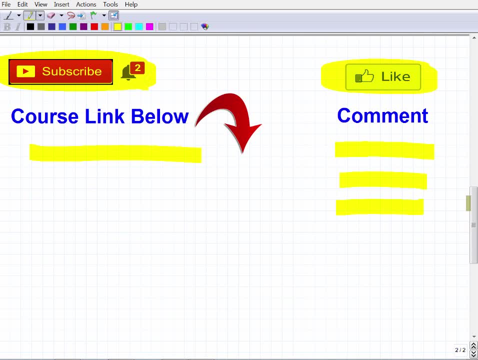 high school doesn't make a difference. You know, don't underestimate the success of the program. There's a lot of test. you know, these assessments to get your certification. you know it's a lot, but that's what we have to do as teachers is, you know, kind of prove our, our skills if you will, so they. 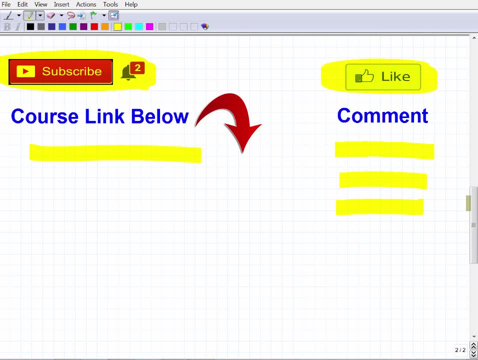 can you know we're we're trusted to teach in the classroom if you will, but you know it's a lot of hard work and sacrifice. but being a teacher, you know, comes with huge rewards as well. so you know, if you're new to teaching, you know and you're looking forward to getting out there all I could. 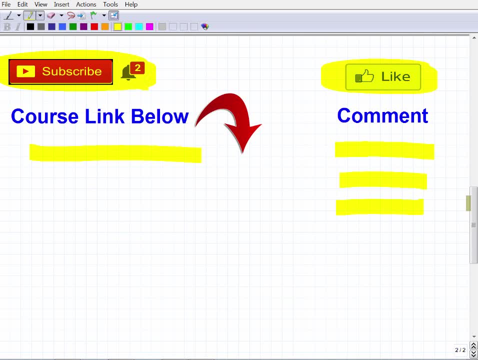 say is: just hey, you know, hang in there while you develop your experience and learn this craft, because over the long run, I think you're, you're really, really will find it a fulfilling- you know- career. you know people don't go into teaching to become wealthy. you know they go in to make 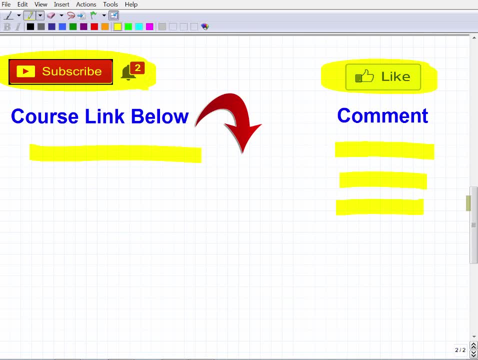 a difference, and we definitely need a great teacher. so I wish you all the best, thank you for your time and have a great day.